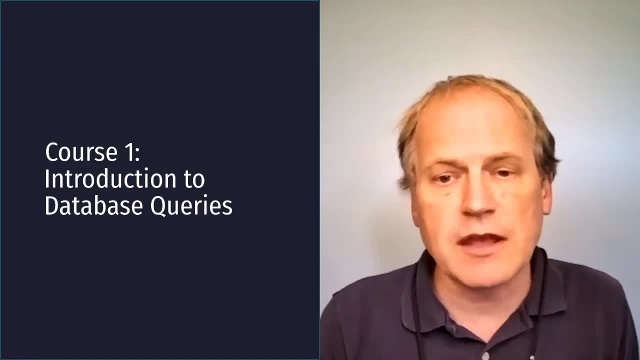 they interact with a commercial database system. We use MySQL in the labs mainly because any student can download it. It runs on almost any platform, So you can run it on Windows, Mac, Linux, So students can download a copy, play with it and then they can submit in. 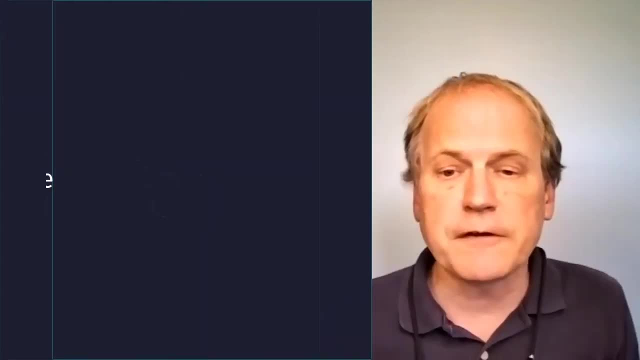 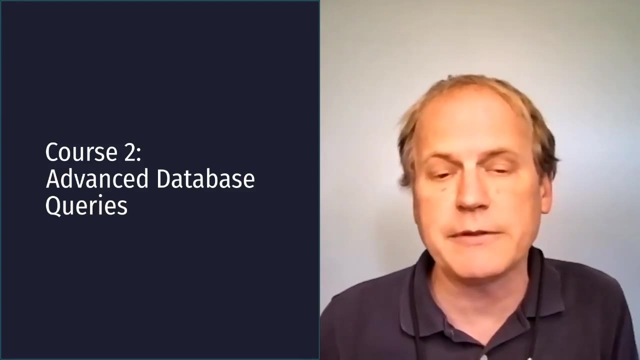 the labs their results to these problems. So in the first course it's really about learning the syntax of this language, And the next course it's really about finding ways to express more complicated queries, Things like aggregates, or using queries inside queries, that sort of thing, And that's a lot of what drives 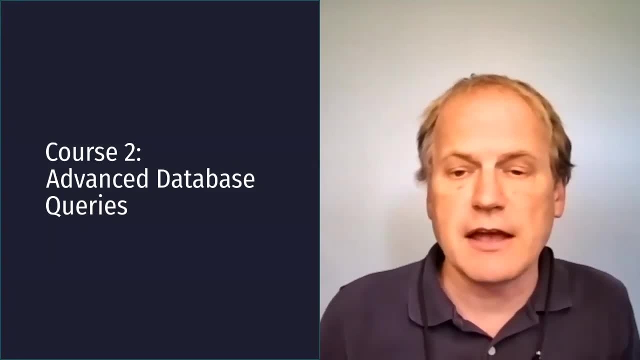 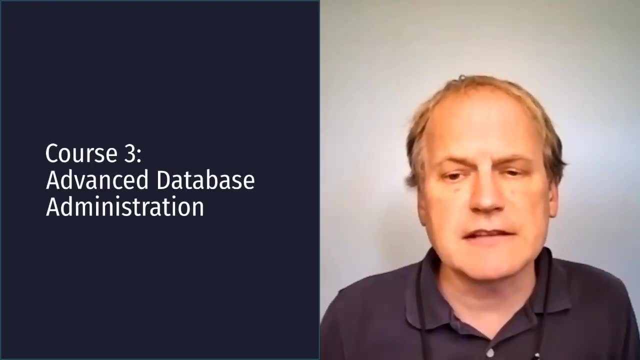 business today, sort of KPIs or dashboards of information, And that's what you're getting in that second part of the database course is how do we express these things? The third course is called Advanced Administration And really in that course we're building 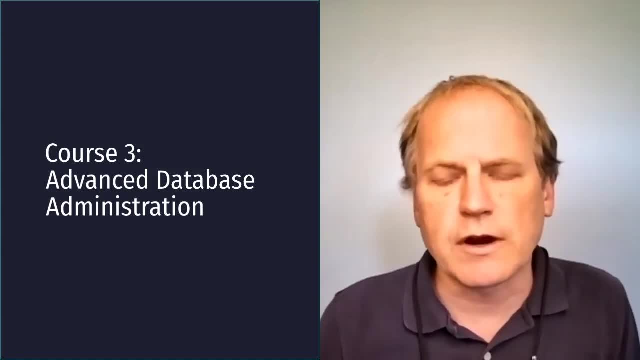 objects in the server that can help us do more work. These can be things like stored programming in the server or views that allow users to see some of the information but not all of the information, And so you can look at the database and say, well, I've. 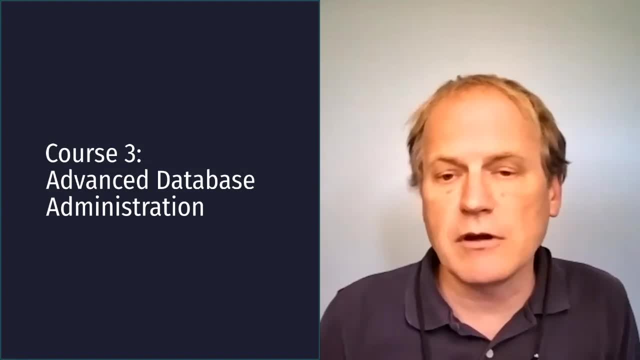 information. So, for example, maybe we've got a payroll table and I want you to see the directory of employees in the company, but not their salary. So that's the kind of things we learned in that third course is how we build objects that others can use, either in applications or interacting. 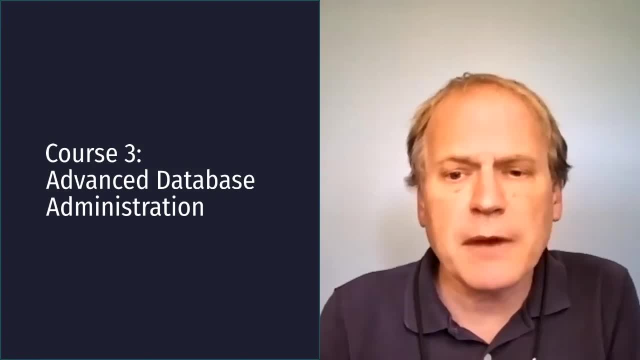 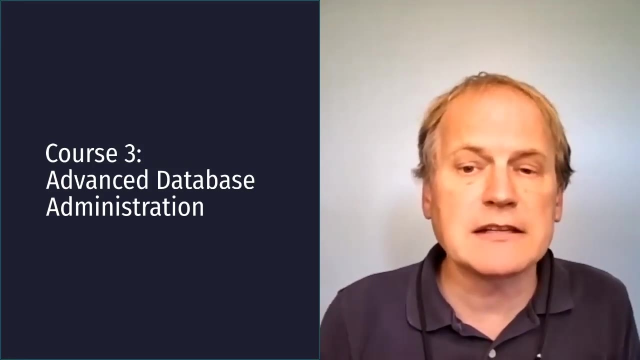 with a database for those first couple courses. But I think the best part is when you walk away with this course you've written 52 successful queries that solve problems, real problems that people have. Now I said we use MySQL, but this applies to lots of other databases. So at the 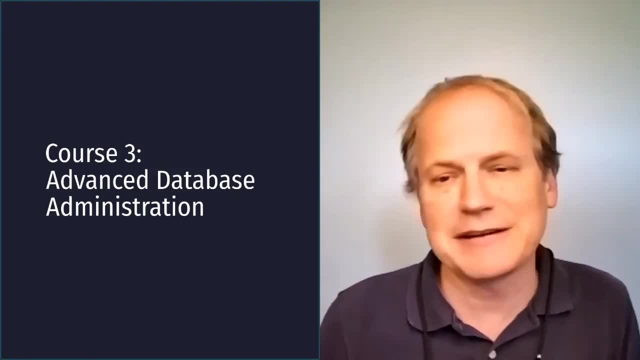 very end of that last course I have a lecture that says other things you need to learn, And it's the things we couldn't get to in a three credits program, but the things that I want you to keep going. So I give you links for reading. So we talk about other commercial databases like 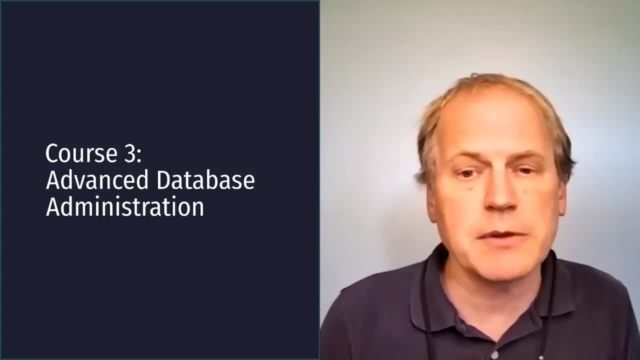 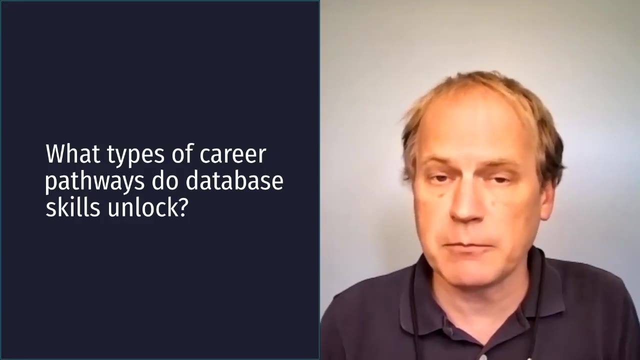 Microsoft SQL and Oracle and IBM DB2 and MariaDB and NoSQL databases. So students really walk away with concrete skills they can use but also knowing where they need to go next. Students with these core skills across these two micro bachelors, programming in a procedural language like Python, networking operating systems.